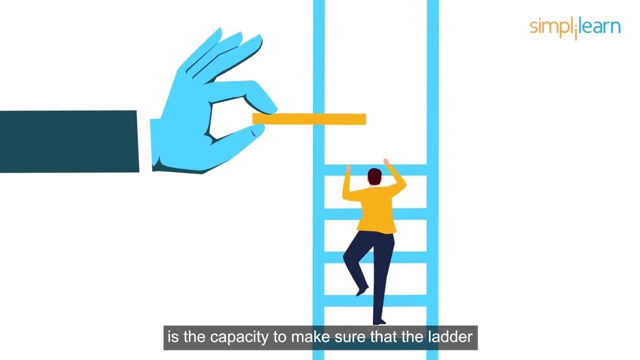 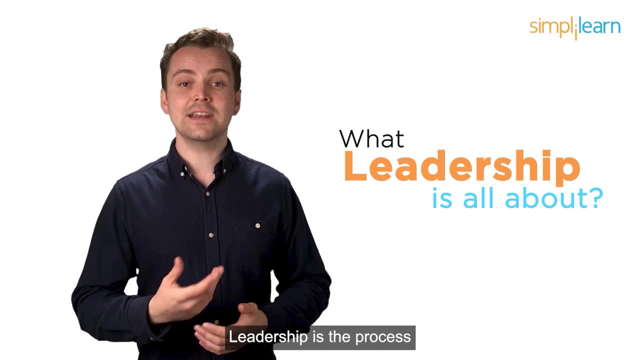 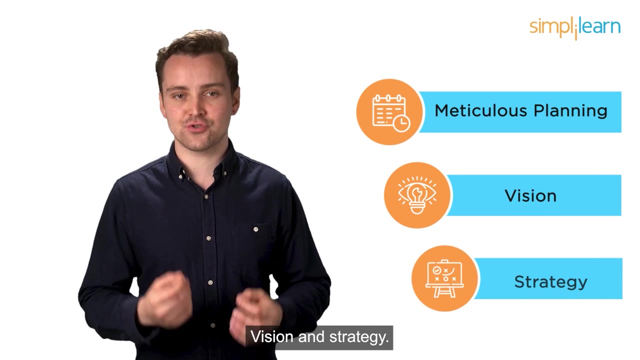 whereas leadership is the capacity to make sure that the ladder is against the right wall Moving forward. let's first understand what leadership is all about. Leadership is the process of driving constructive, non-incremental change through meticulous planning, vision and strategy. 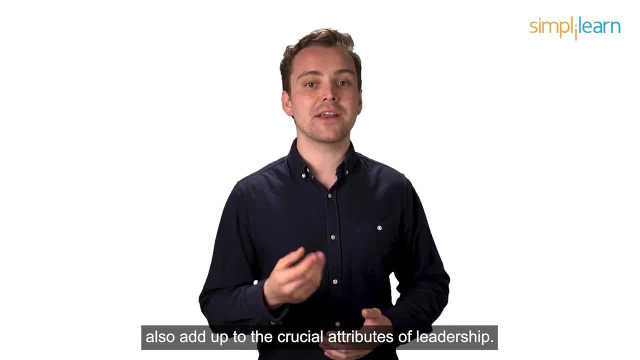 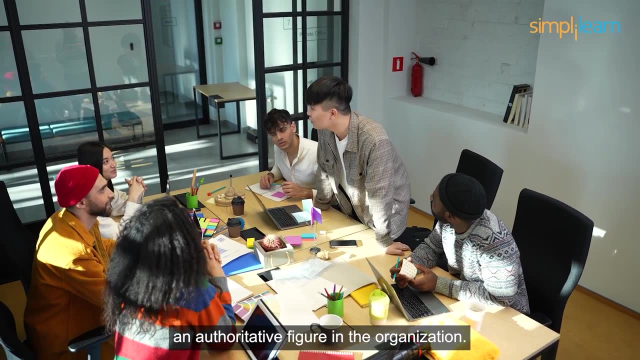 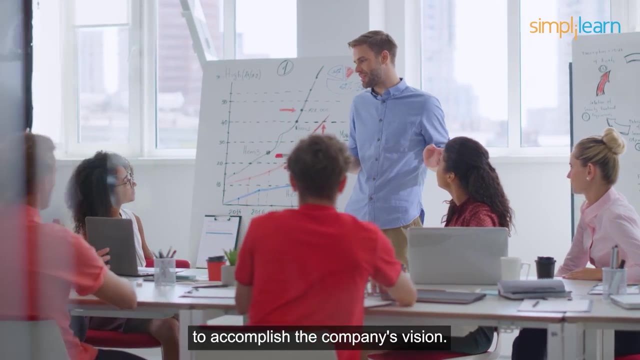 Workforce empowerment and adaptive decision-making also add up to the crucial attributes of leadership. To become a leader, you are not required to hold an authoritative figure in the organization. A leader is someone who always takes the initiative and invests a great effort to accomplish the company's vision. 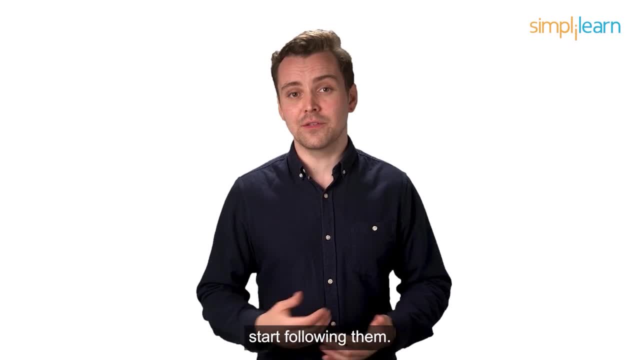 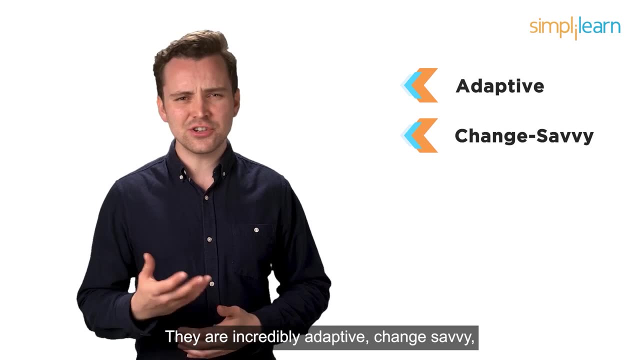 That is the only reason why people around start following them. Leaders in general are those who question the status quo. They are incredibly adaptive, change savvy, visionary, agile and creative. We have a dedicated video on leadership skills. Here's a video link to that. 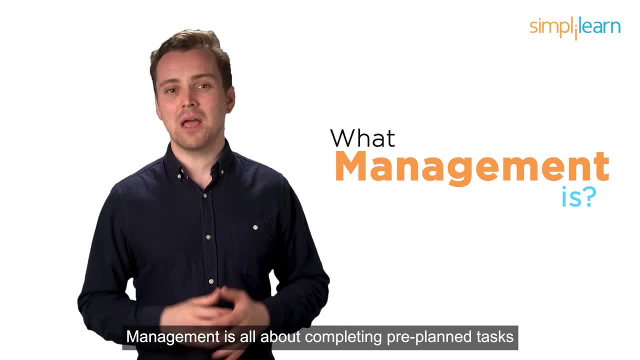 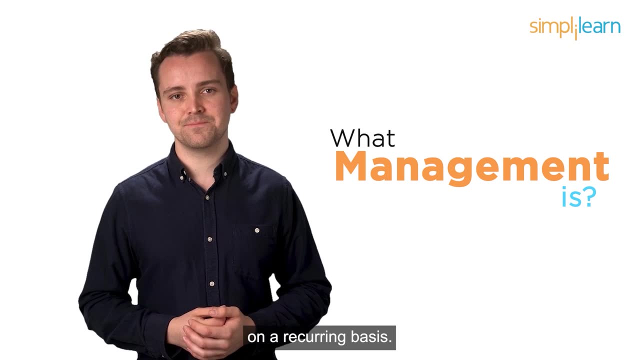 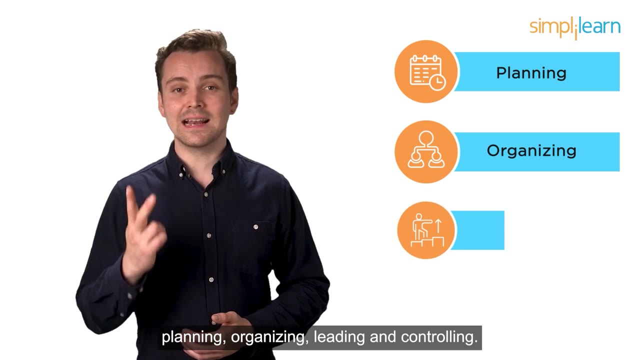 Now let us understand what management is. Management is all about completing pre-planned tasks with the support of your team. A manager is completely responsible to carry out the four important functions of management – planning, organizing, leading and controlling. Managers can become leaders if they adequately. 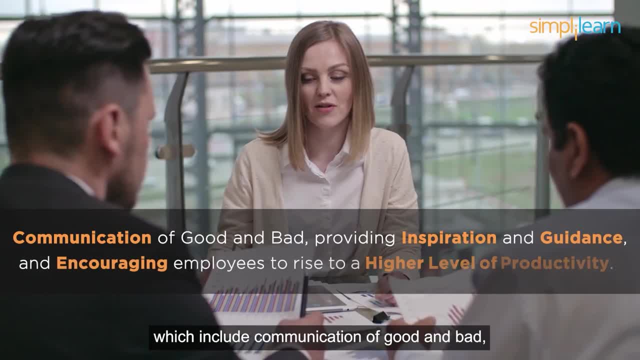 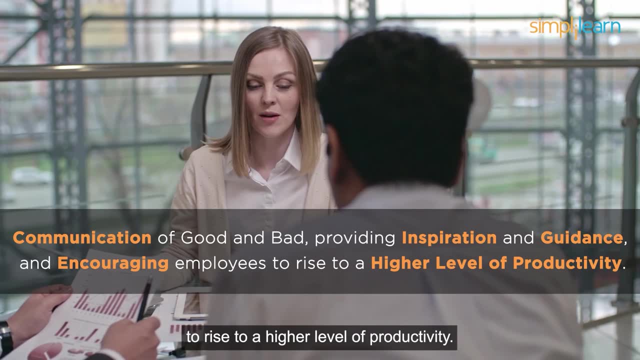 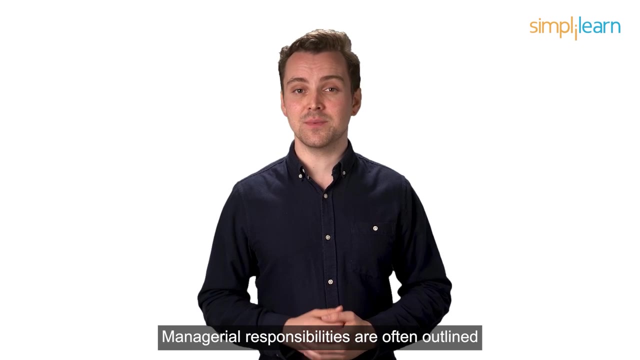 carry out leadership responsibilities, which include communication of good and bad, providing inspiration and guidance and encouraging employees to rise to a higher level of productivity, But unfortunately, not all managers can achieve that. Managerial responsibilities are often outlined in a job description. 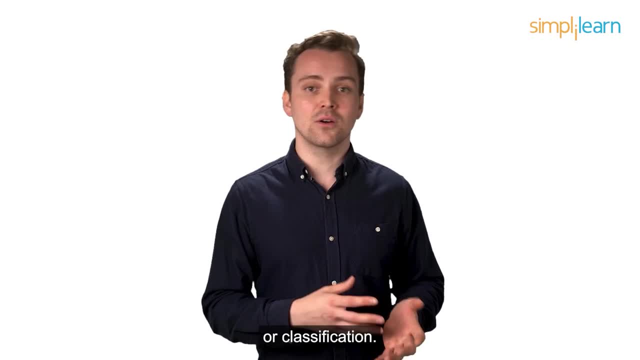 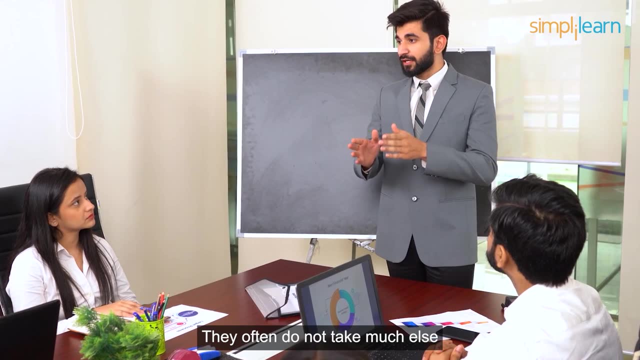 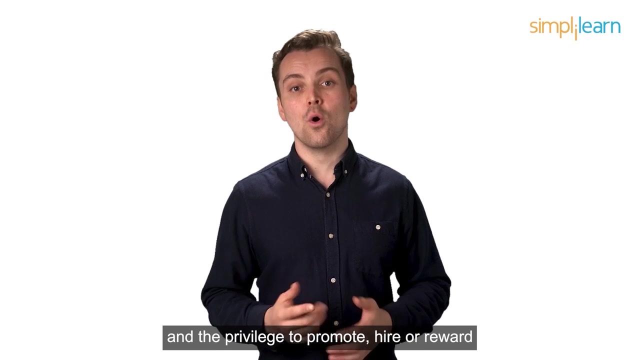 with subordinates following because of the professional title or classification. A manager's primary focus is meeting organizational goals. They often do not take much else into consideration. With the title comes the authority and the privilege to promote, hire or reward employees based on their performance. 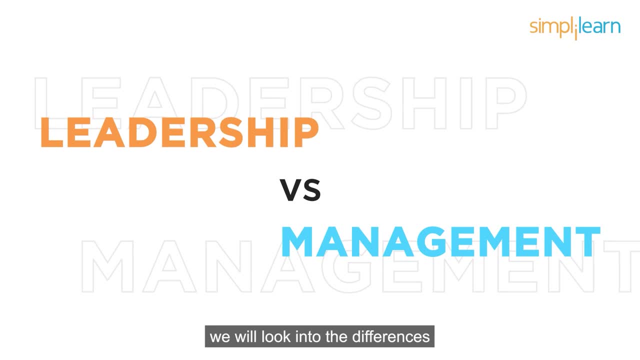 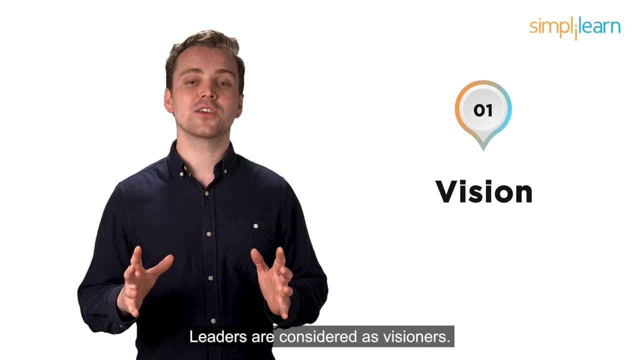 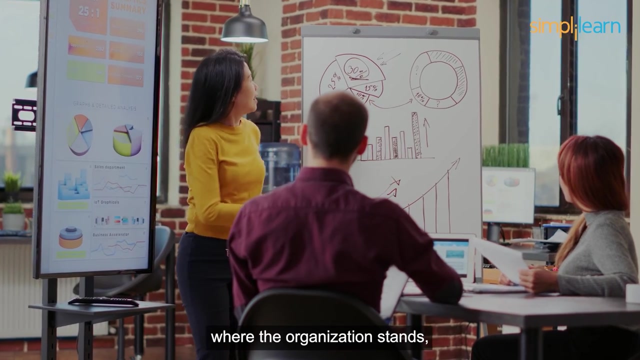 and behavior. Moving ahead, we will look into the differences between leadership, leadership and management. The first area of difference is vision. Leaders are considered as visioners. They set the path to excel the organizational growth. They always examine where the organization stands, where they want. 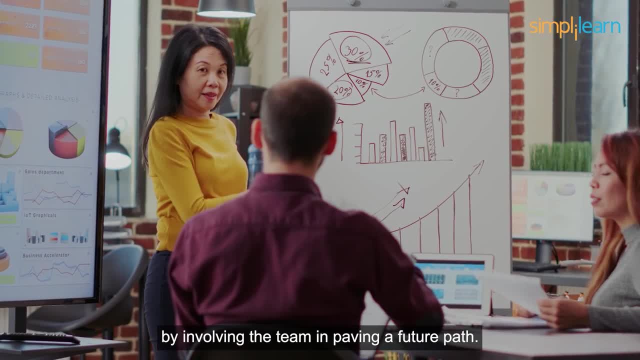 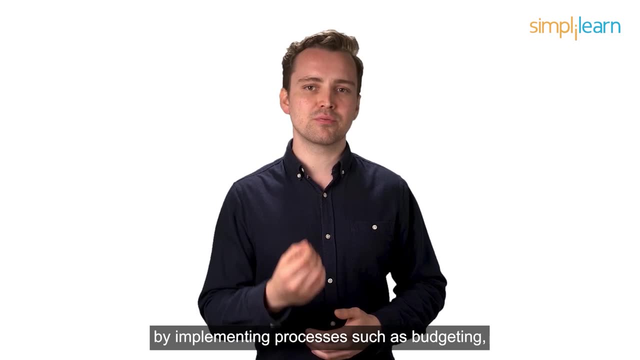 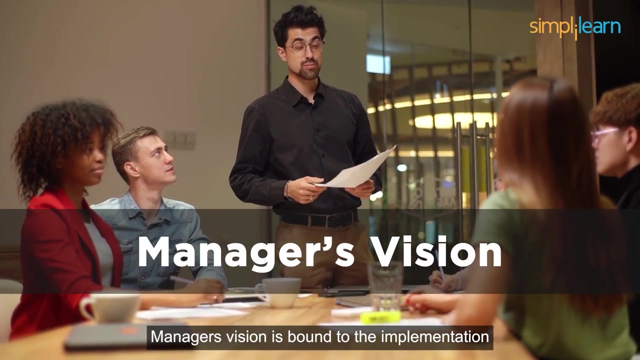 to go and how they can reach there, by involving the team in paving a future path. In comparison, managers set out to achieve organizational goals by implementing processes such as budgeting, organizational structuring, staffing managers. vision is bound to the implementation, strategies, planning and 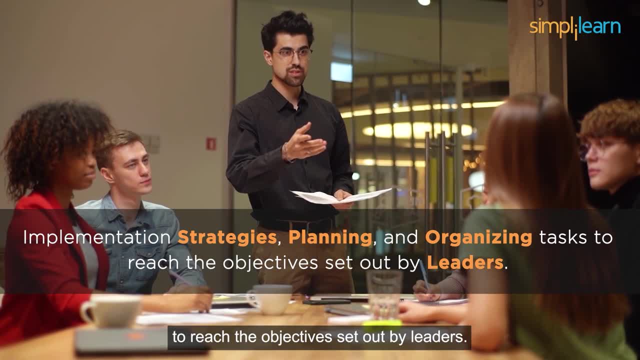 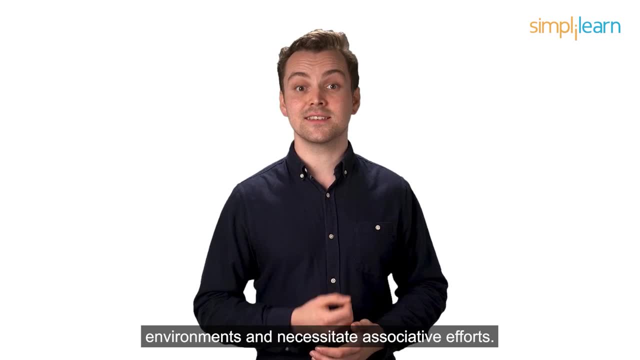 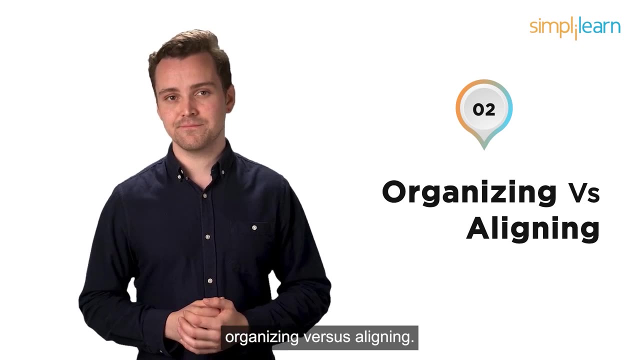 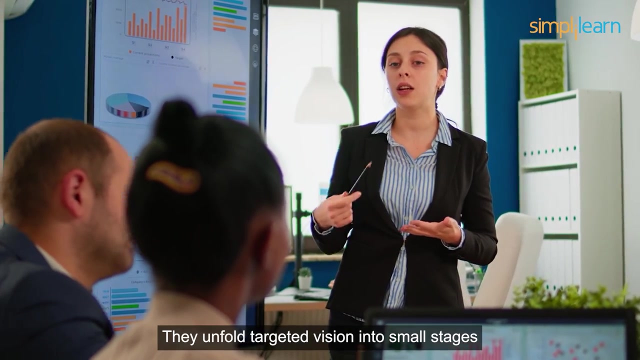 organizing tasks to reach the objectives set out by leaders. however, both of these roles are equally important in the context of business environments and necessitate associative efforts. the next field of differentiation is organizing versus aligning. managers pursue objectives through coordinated actions and tactical processes. they unfold targeted vision into small stages and 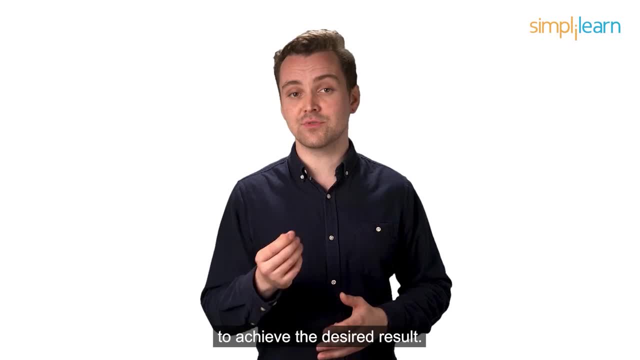 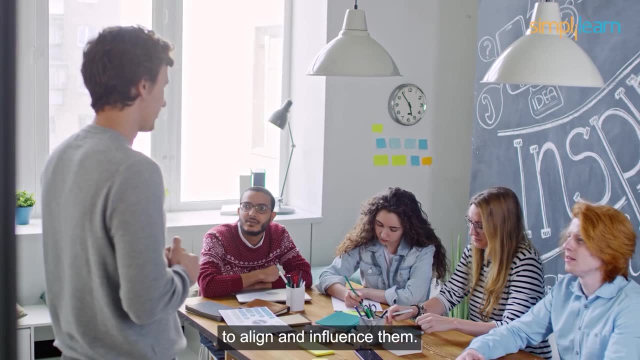 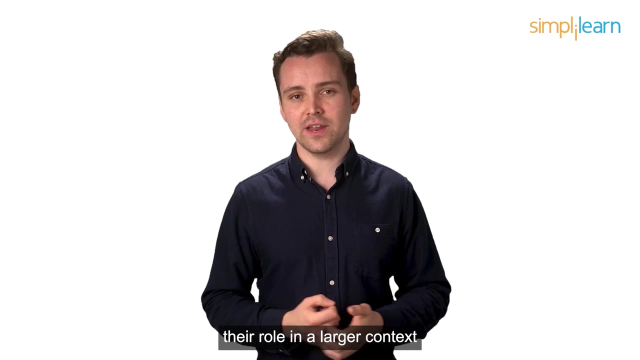 organize available resources to achieve the desired result. leaders, on the other hand, are less focused on how to organize people and more on finding ways to align and influence them. they accomplish this by helping individuals envision their role in a larger context and the future growth potential their efforts can. 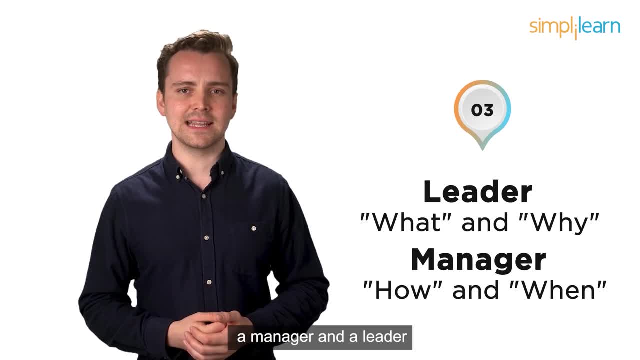 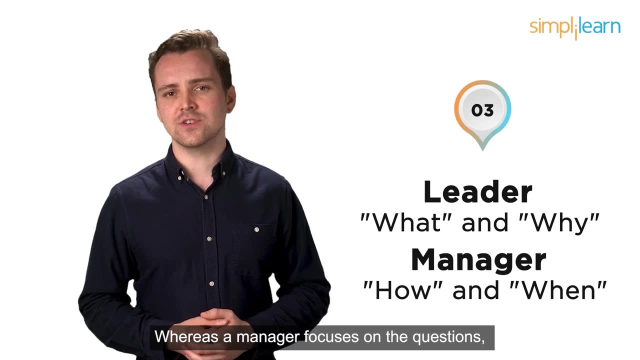 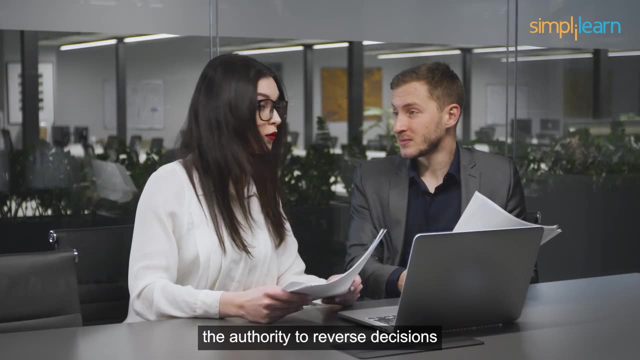 provide. the third distinction between a manager and a leader is that a leader asks the questions what and why, whereas a manager focuses on the questions how and when to do justice to their duties. as a leader, one might question and challenge the authority to reverse decisions that may not be in the 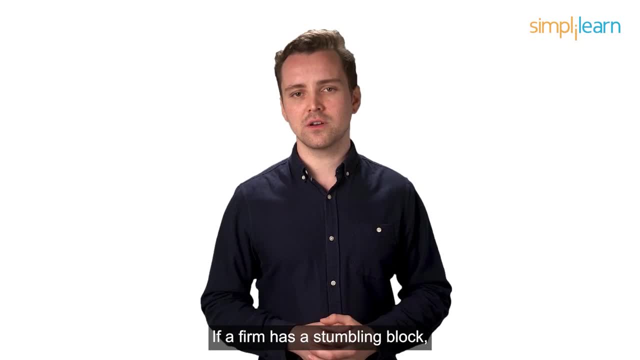 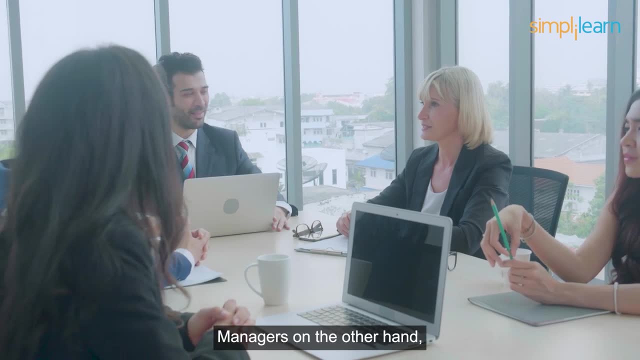 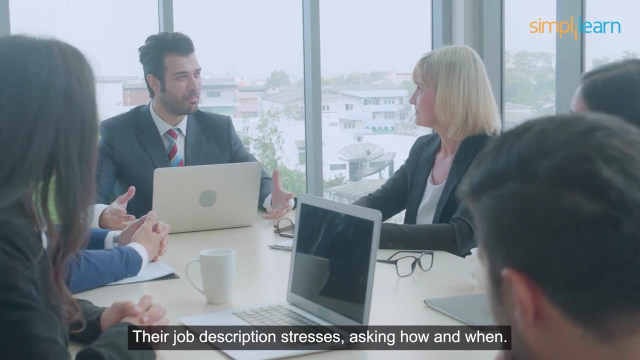 better interests of the team. if a firm has a stumbling block, a leader will be the one to step up and ask: what did we learn from this and why has this happened? managers, on the other hand, are not compelled to evaluate failures. their job description stresses asking how and when which helps them. 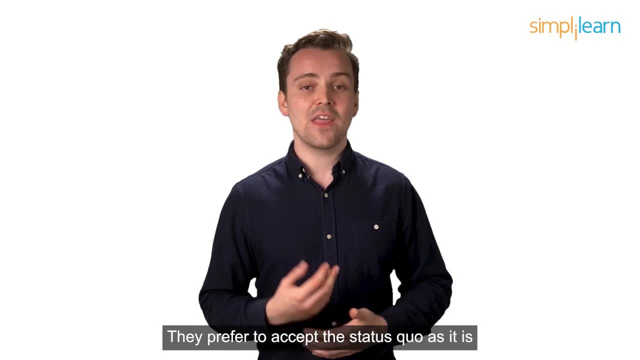 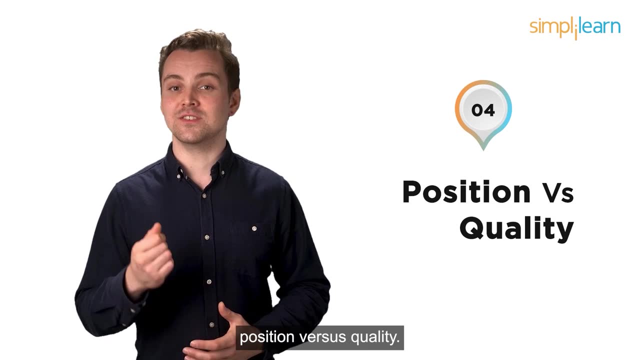 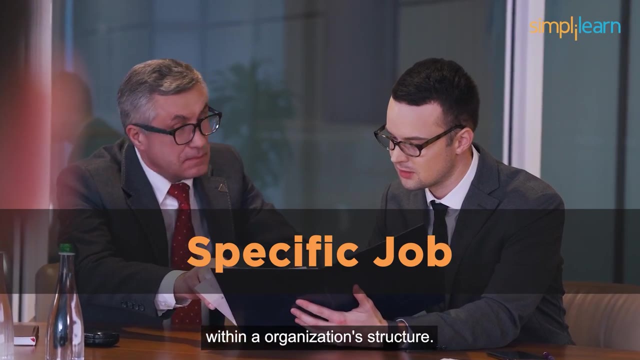 ensure that plans are carried out appropriately. they prefer to accept the status quo as it is and do not strive to change it. the final factor on our list is position versus quality. a manager is a role that frequently refers to a specific job within a organization structure, whereas the term leader has a. 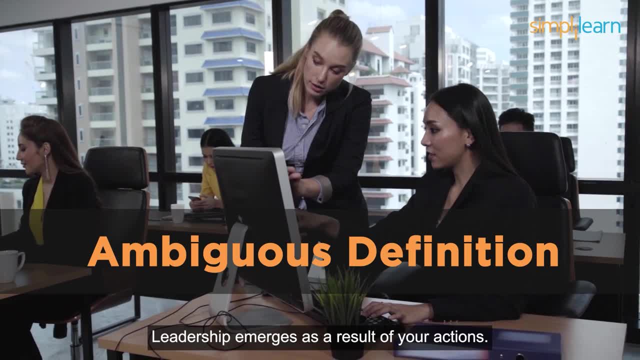 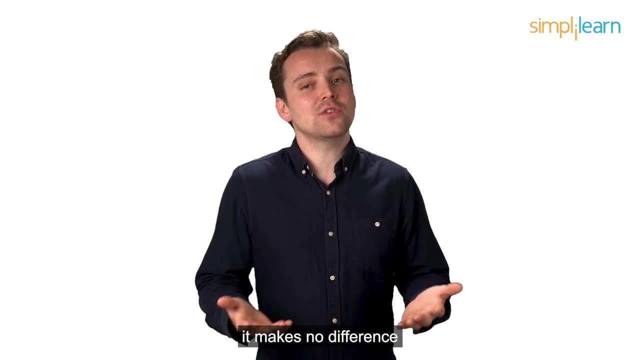 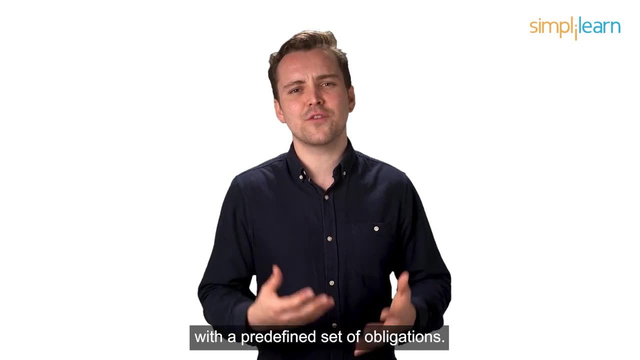 more ambiguous definition. leadership emerges as a result of your actions. if you are a leader and act in a way that inspires others to do their best, it makes no difference what your title or position is. a manager, on the other hand, is a job title that comes up with a predefined 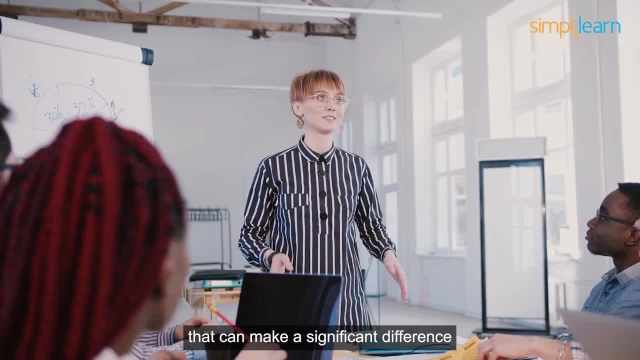 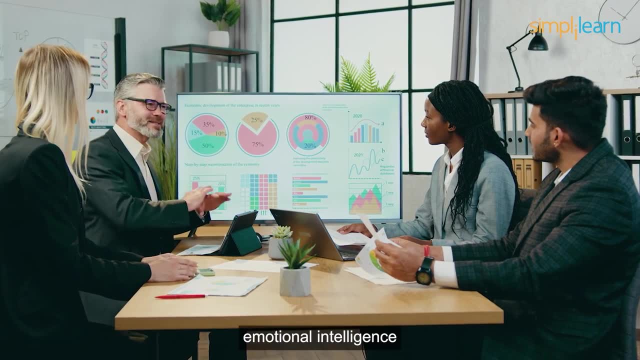 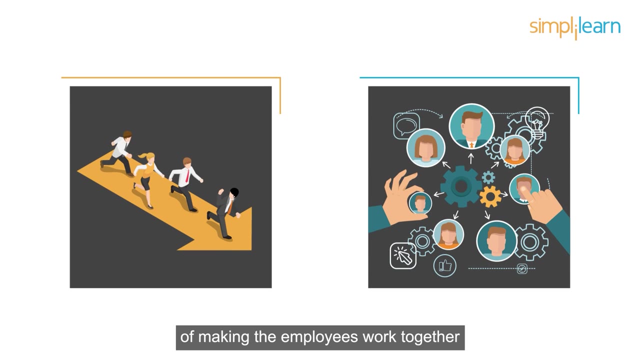 set of obligations. leadership is a great quality that can make a significant difference in your respective careers, and with passing time you can shape it by developing emotional intelligence and learning how to influence others. leading and managing are two contrasting ways of making the employees work together more efficiently.